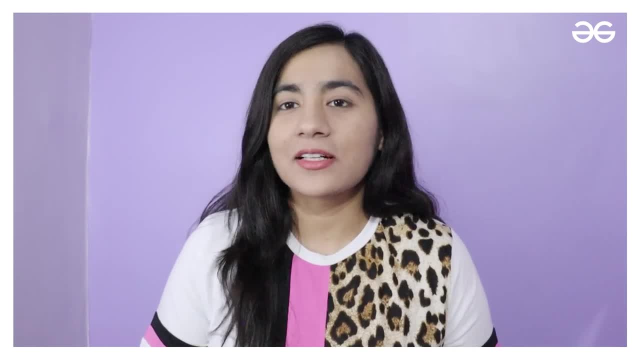 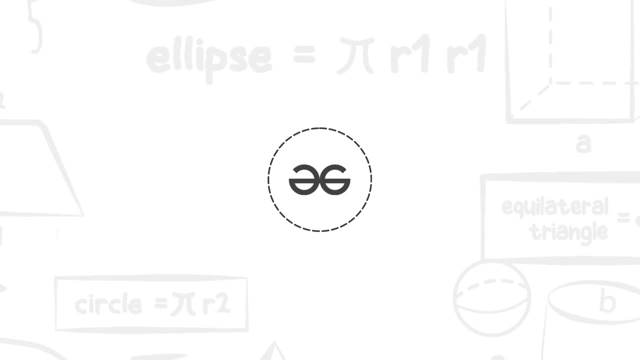 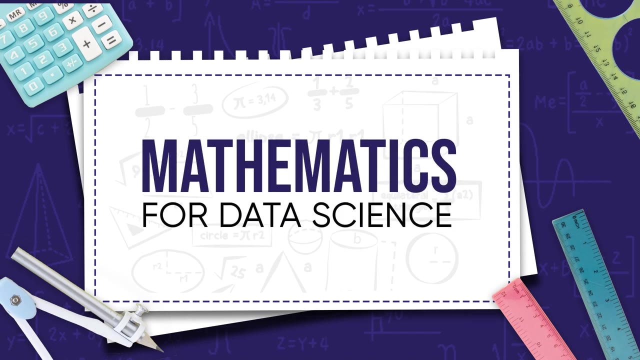 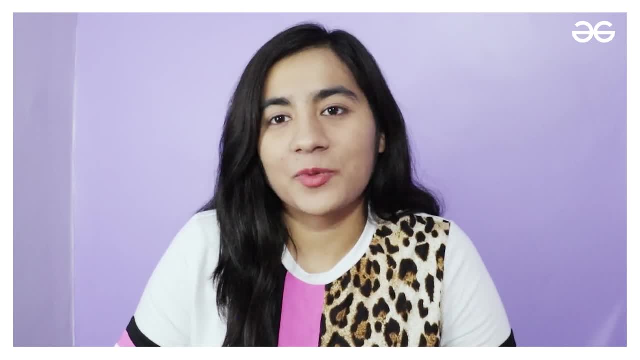 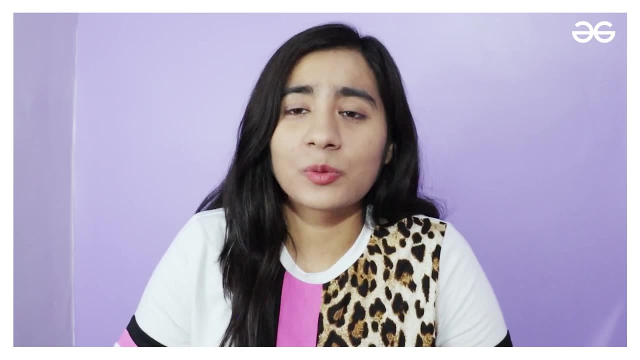 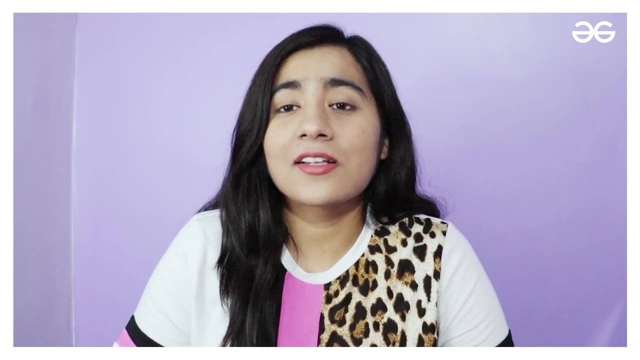 Mathematics is the heart of machine learning algorithms. You may have applied it using Python libraries like scikit-learn, But have you ever wondered, like how these algorithms work internally, How the final result is being calculated? When you study machine learning in depth, then you will get to know that there's a lot of math involved in producing the final result. 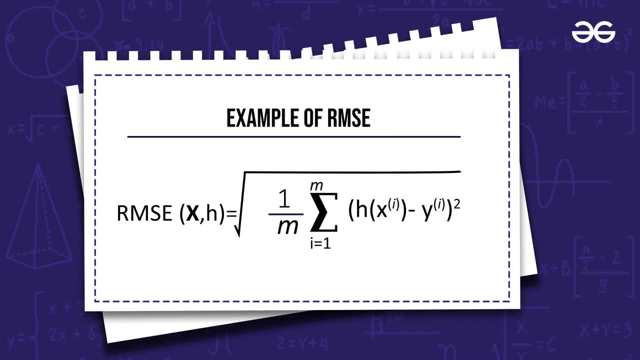 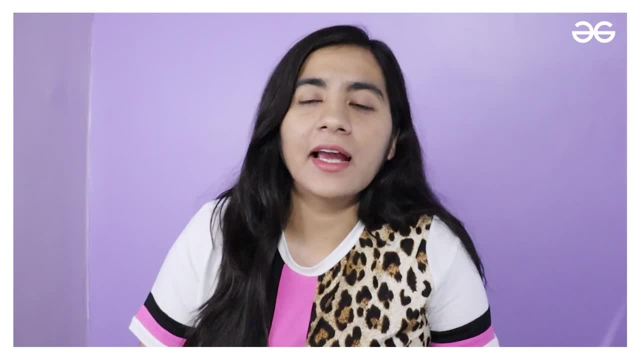 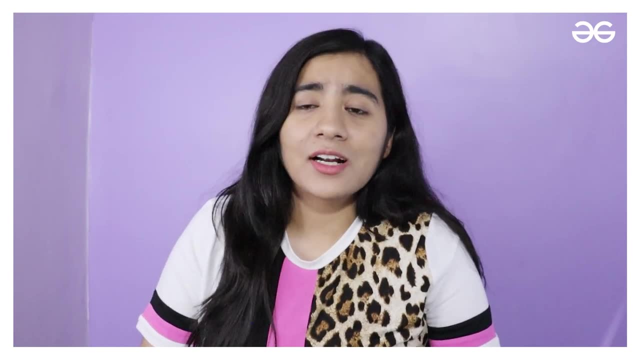 If we take example of RMSE, root mean square error is the preferred performance measure of regression models. Now RMSE measures the distance between the vector of predictions HXI and vector of target labels YI. It is the root of sum of squares of these distances. How do we do this? on large arrays of data? All thanks to vector and. 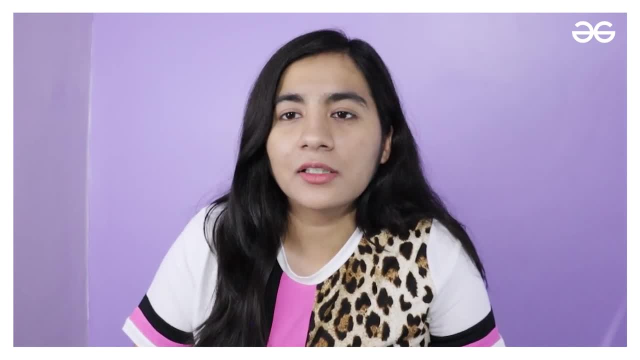 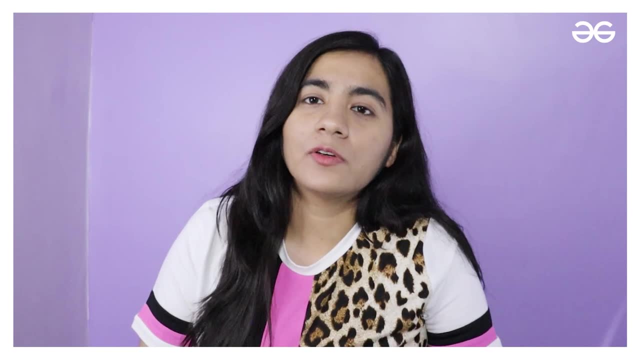 linear algebra. Now I hope with this example it's a little bit clear to see mathematics as a part of data science. Let's just start with the fields of mathematics that you're going to encounter while working on different algorithms in data science and where you will be using them. First, let's just 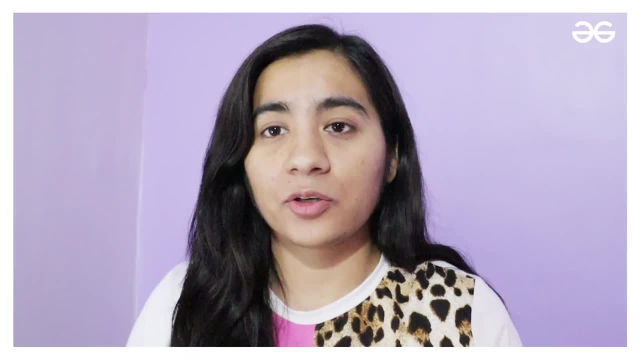 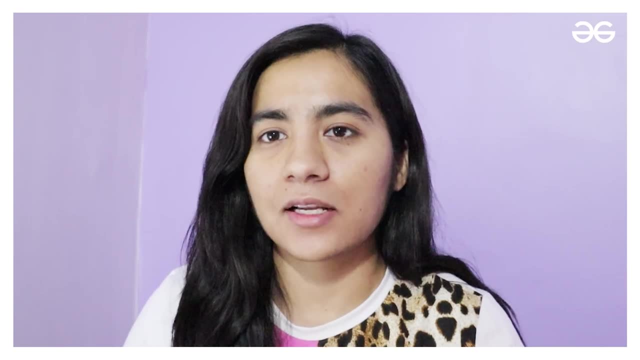 start with basic mathematics. So if you have opted for basic mathematics, then you will be able to use them. If you have opted for maths in your 11th or 12th grade, you must be familiar with these concepts. You just need to recall them and see their implementation in your data science algorithm. 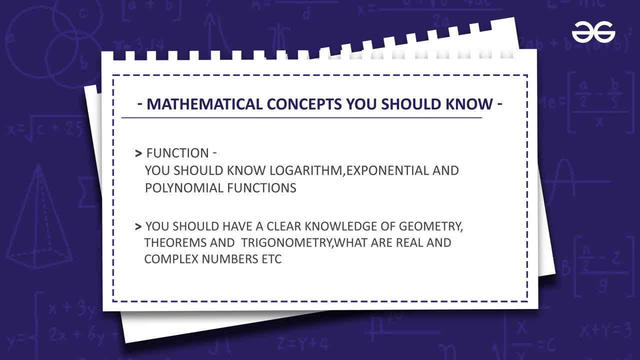 Some of the mathematical concepts are like functions. You should be familiar with what is logarithmic function, exponential function, polynomial function. And the second point is like you should be familiar with basic theorems, geometry, trigonometry. and then what is real? 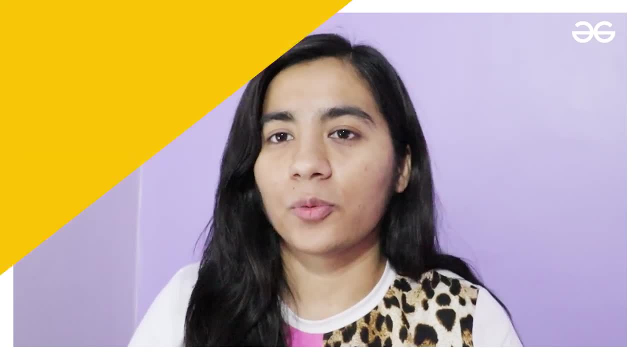 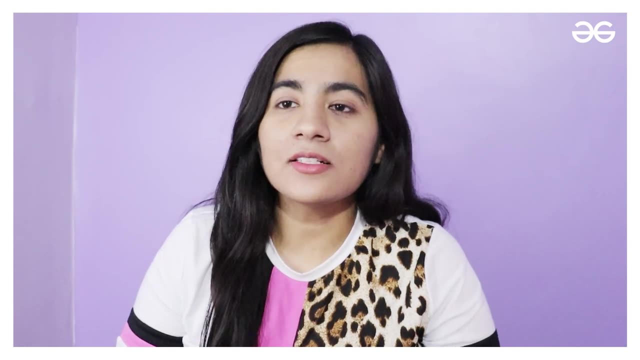 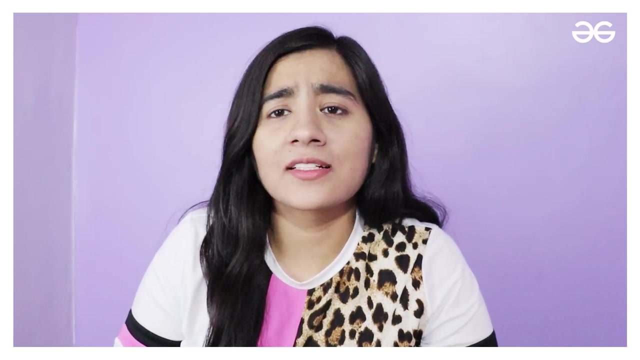 number, what is complex number, etc. And then you're good to go. Second is statistics. Why is this important? Statistics allow us to drive knowledge from large data sets, and then this knowledge can be used to make predictions, decisions and classifications. Many companies are using statistics, like Netflix. 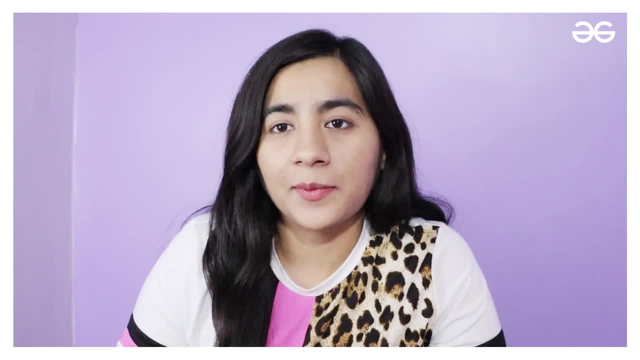 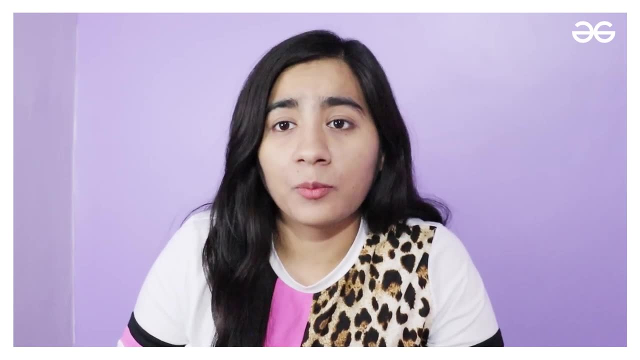 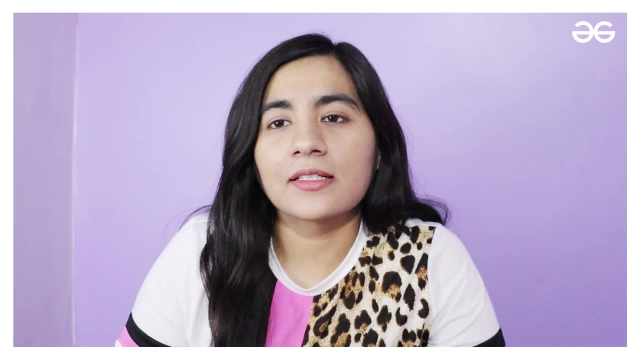 Amazon, Prime, Hotstar. These companies are using movie recommendation systems where they do statistical analysis to gather what kind of movies you like, what kind of movies people like, your age, your background like, and then they recommend you movies and TV shows. You can also use statistics in 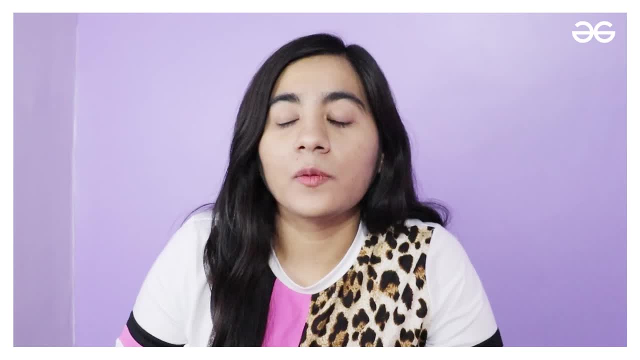 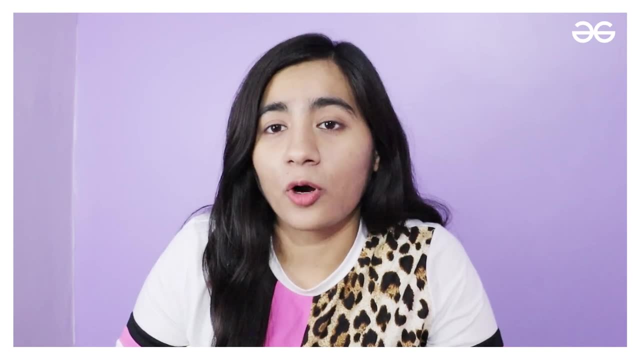 classification and time series analysis, You can analyze what will be the price of a stock in the upcoming days. Now, these results are not 100% accurate and they might give you some wrong predictions as well. Statistics is about making a decision based on current trends. It tells you. 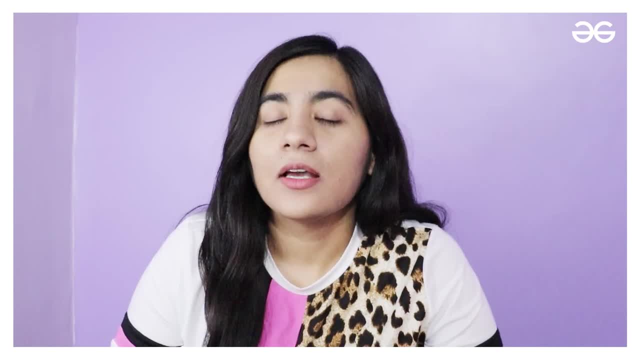 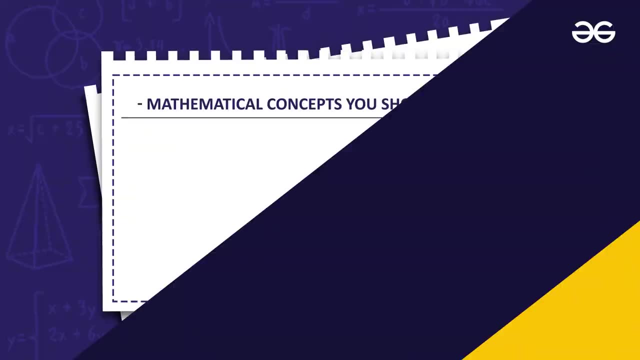 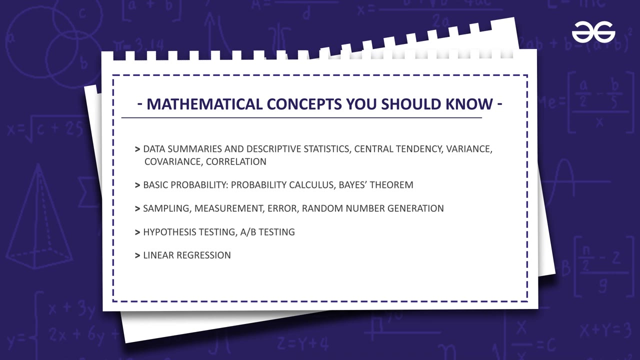 what should be done based on these particular data. Statistics is used in projects like medical research, stock market analysis, sales projection and weather forecasting- Mathematical concepts you should be familiar with. First one is data summaries and descriptive statistics. central tendency variance. 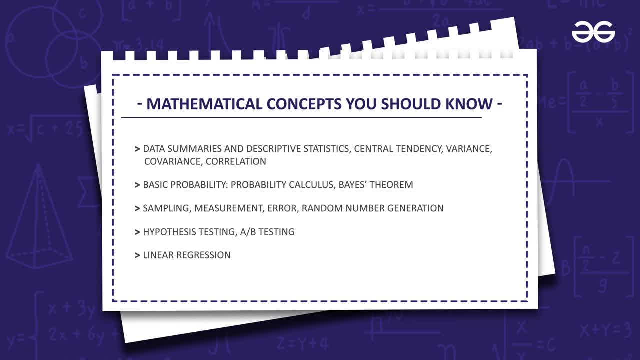 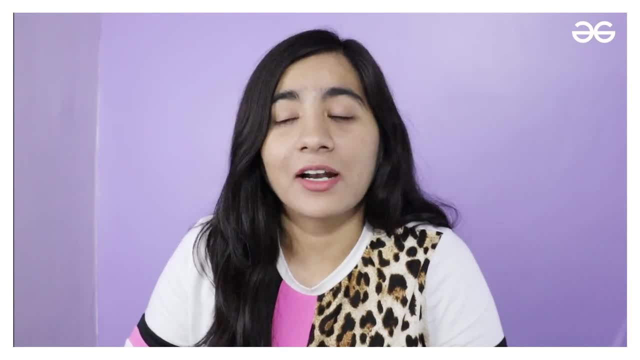 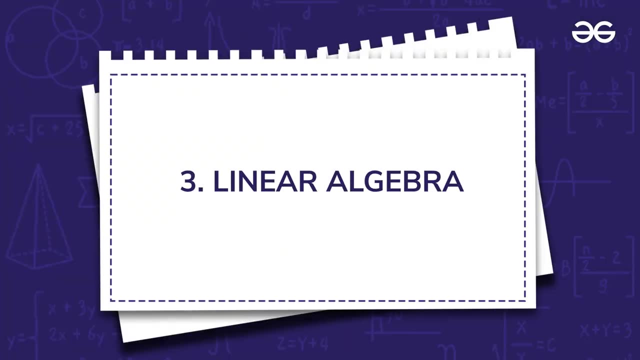 covariance, correlation, basic probability concepts, calculus, Bayes theorem, Then you have sampling, you have measurement, you have error, you have random number generation, then hypothesis testing, A-B testing and finally linear regression. Third one is linear algebra. Now it's really hard. 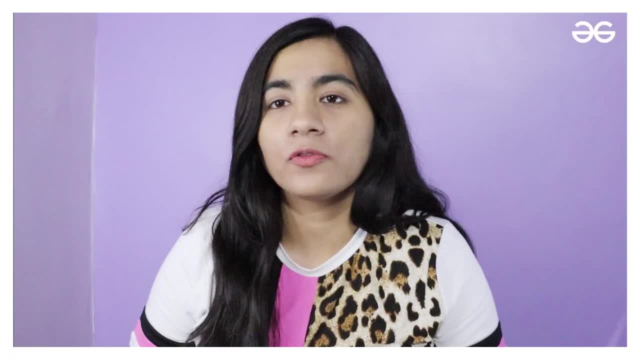 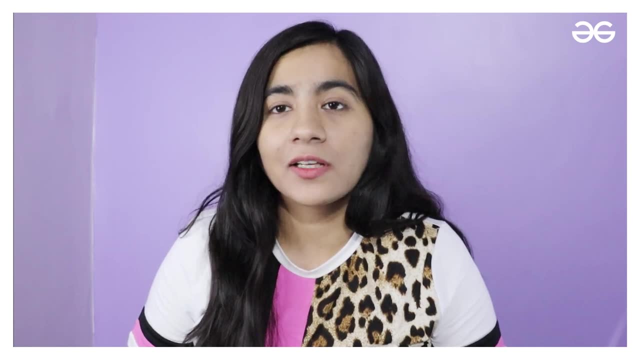 to imagine data science without linear algebra. It is used in a lot of algorithms, but you don't have to go in deep with these concepts. It is not expected from you to write them with your hands while solving a data science problem, but you should be familiar with like how the things work. 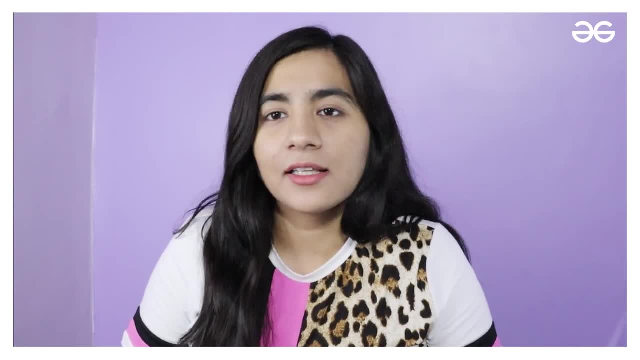 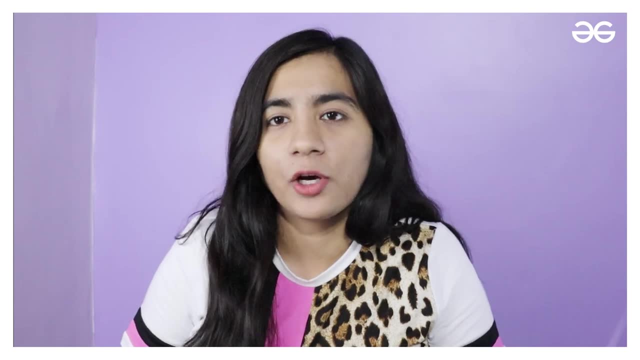 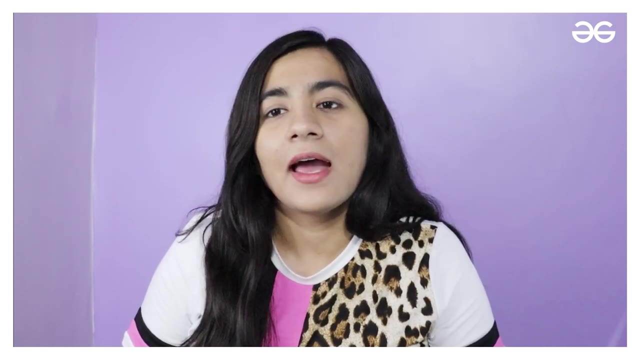 under the hood so that you can make changes here and there and get the desired results. You already have used linear algebra, if you have performed principal component analysis to reduce the dimensionality of your data. All neural network algorithms use linear algebra techniques to represent and process network structures and learning operations- Topics you should be familiar. 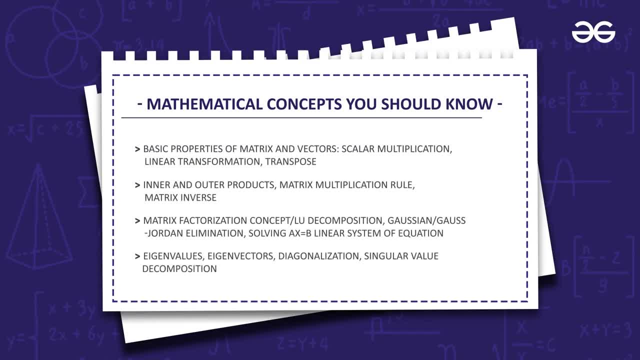 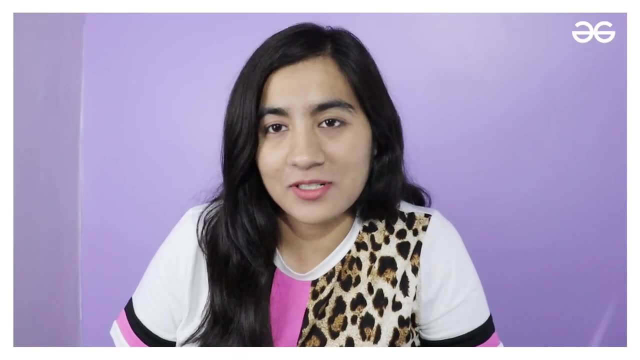 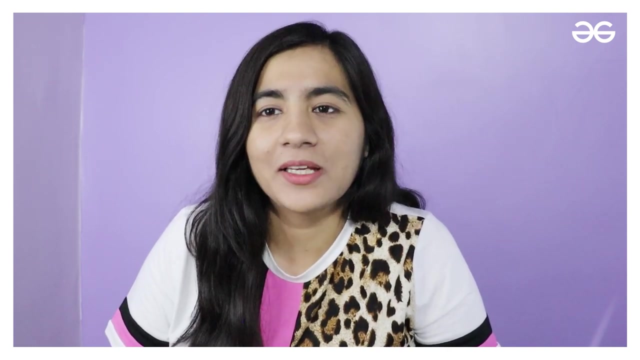 with are basic properties of matrix and vectors like scalar multiplication, linear transformation, transpose. Second one is inner and outer products: matrix multiplication rule, matrix inverse. Third one is matrix factorization concept, LU decomposition, Gaussian, Gauss-Jordan elimination, solving AX equals to B, linear system of equation. So these are the concepts that you have to make. 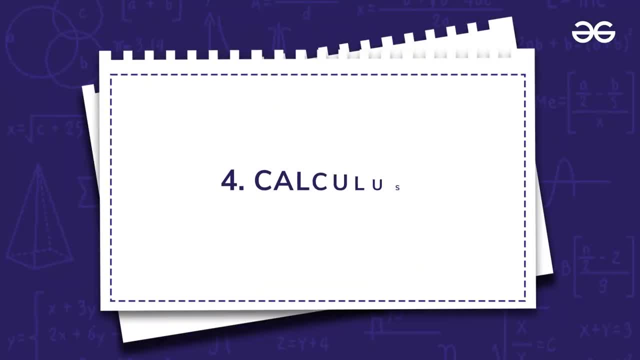 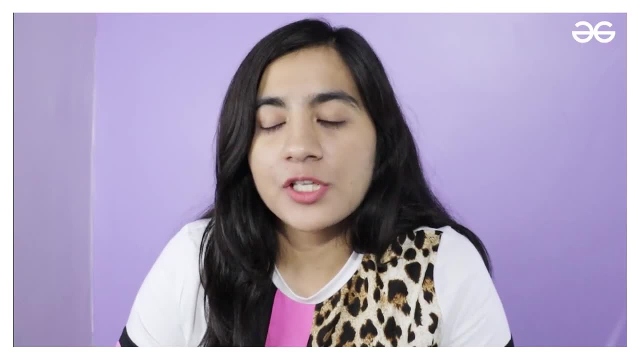 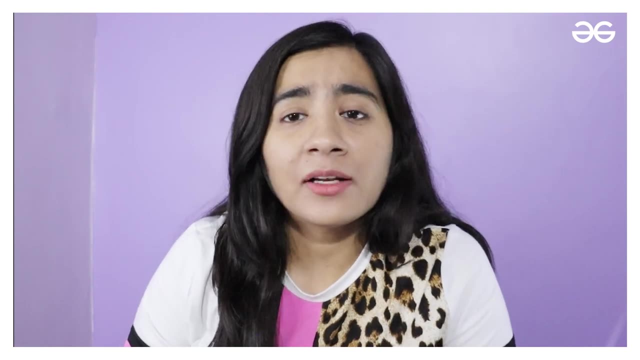 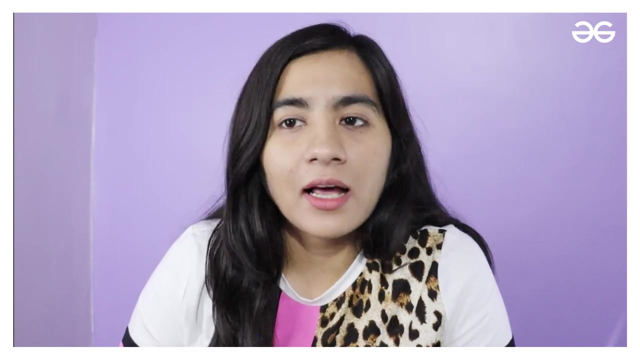 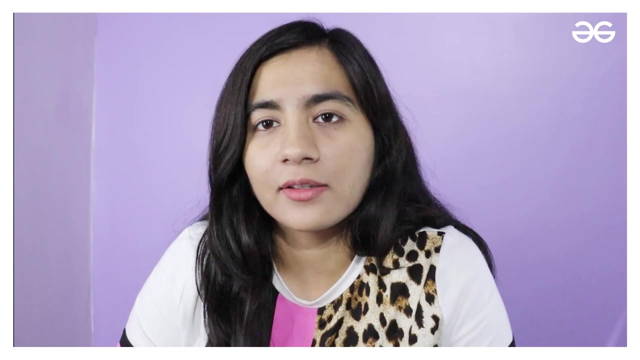 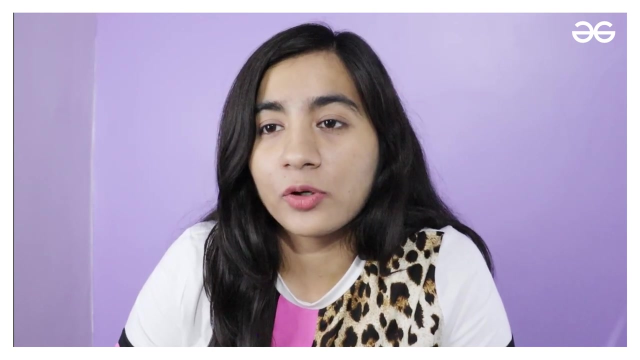 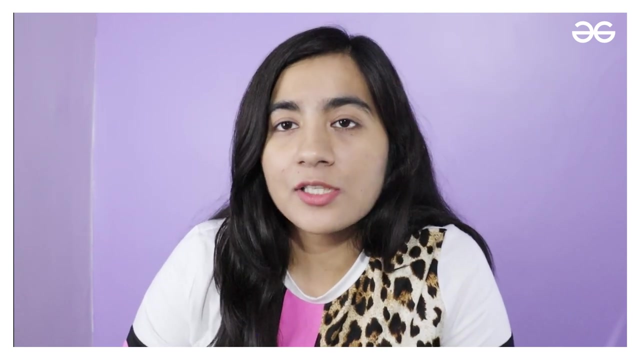 yourself familiar with. Thank you very much for watching this video. If you have any questions, feel free to ask them in the comment section below. Calculus, as I said before, is used for most every algorithm in machine learning. A basic example that you must be familiar with is gradient descent. Gradient measures. the output changes if you 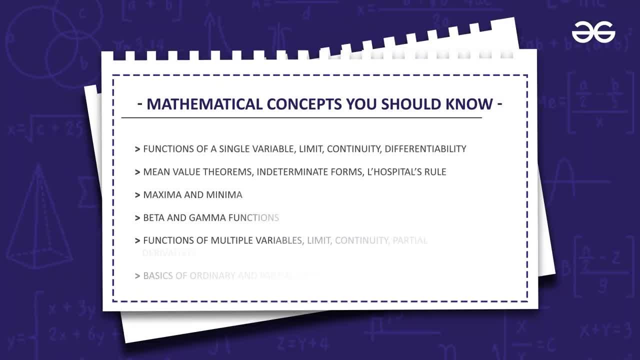 change the inputs a little bit. The topics that you should be familiar with are fixed functions of a single variable, like limit, continuity, differentiability, mean value theorem, indeterminate forms, LHTML, and so on, So be prepared to learn from these concepts if you are new to the course. 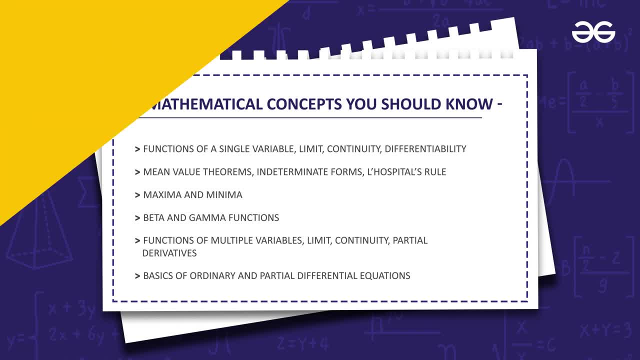 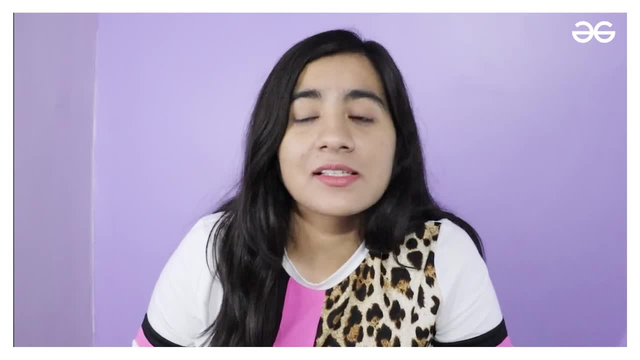 In this video we are going to talk about a few basic parameters of machine learning. First we l hospital rule: what is maxima and what is minima? third one is beta and gamma functions. fourth one is functions of multiple variables: limit continuity, what is partial derivatives and 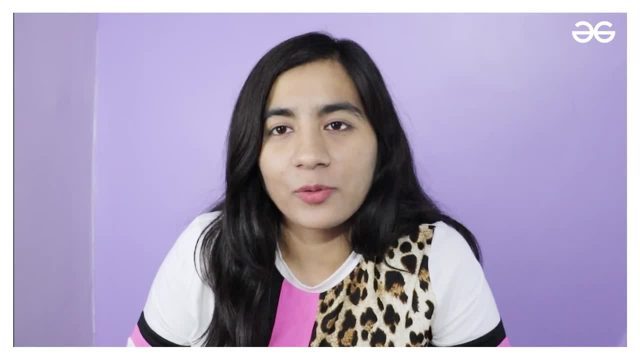 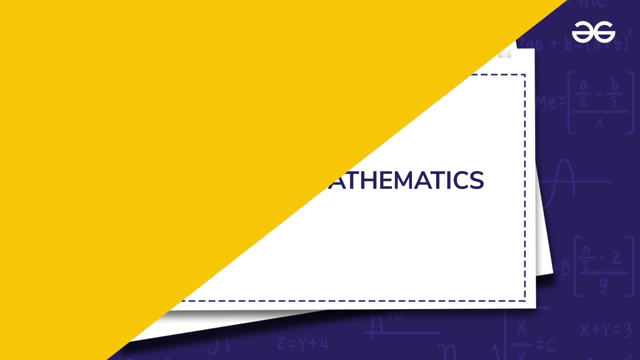 finally, basics of ordinary and partial differential equations. finally, i want to talk about our fifth point, that is, discrete math. now, if you're from an engineering background, you must have gone through this subject in your first year or second year, and it was pretty easy to understand and solve. 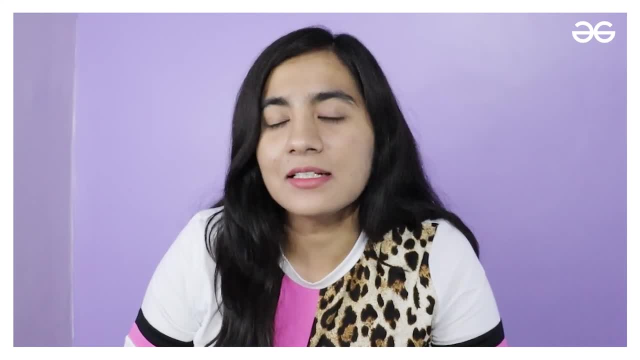 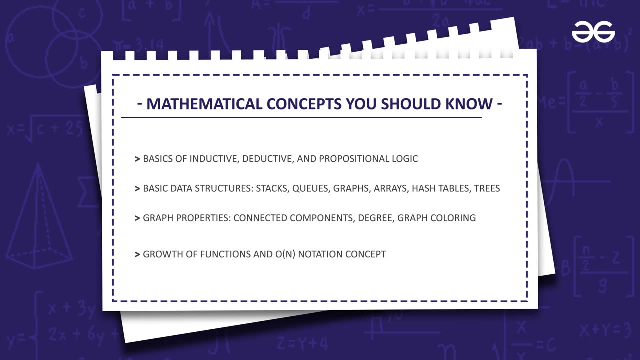 here we work with sets, subsets, basic proofing techniques like induction, proof by contradiction. then we work with basics of inductive, deductive and propositional logic. we have seen the data structure concepts like stacks, queues, graphs, arrays, hash tables. then we have worked with graph properties like what is connected, components, what is the degree and what is graph coloring. 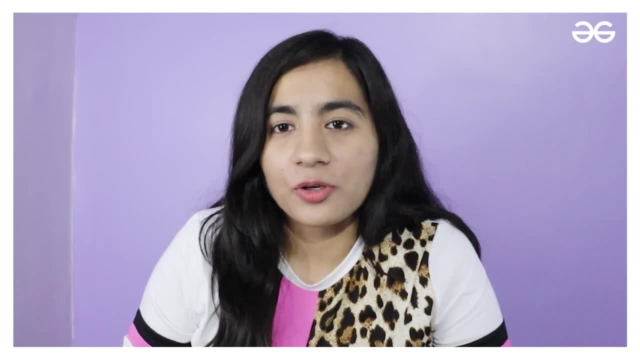 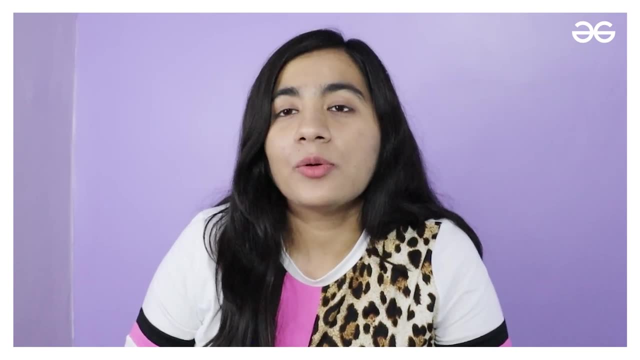 then, finally, we cover the basic proofing techniques, like induction proof by contradiction. then we work with this, with o and notation concepts. now, this will be used in knowing how the system change when you increase the input data size. you need to understand what is the time and space complexity, basically by